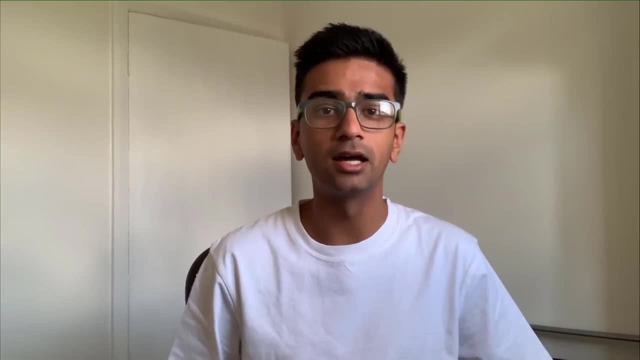 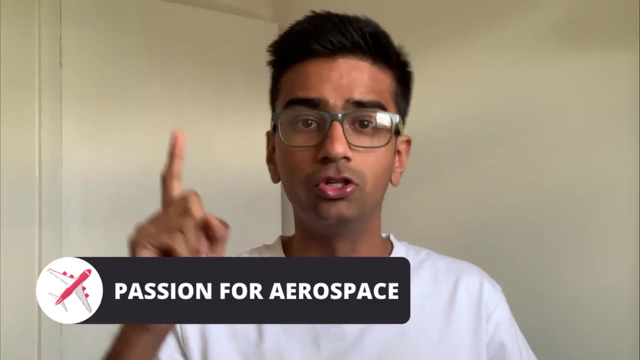 Studying aerospace engineering at university is not for everyone, and in this video I'm going to share five traits that I think suggest that you should study aerospace engineering. Point one: you have a passion for aerospace. If you already have a strong passion for aircraft and spacecraft. 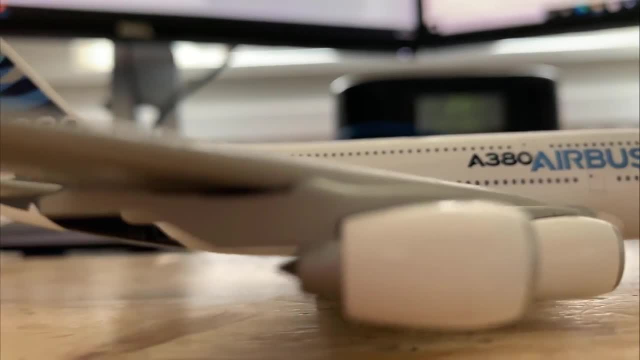 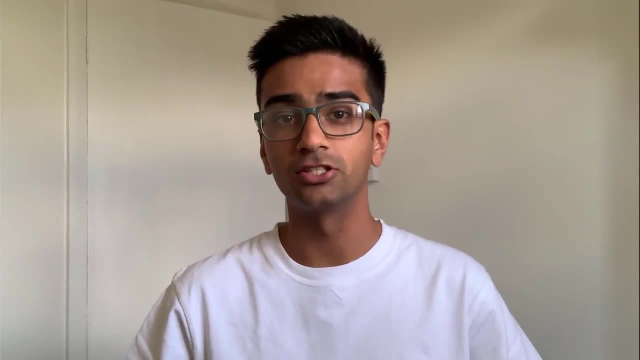 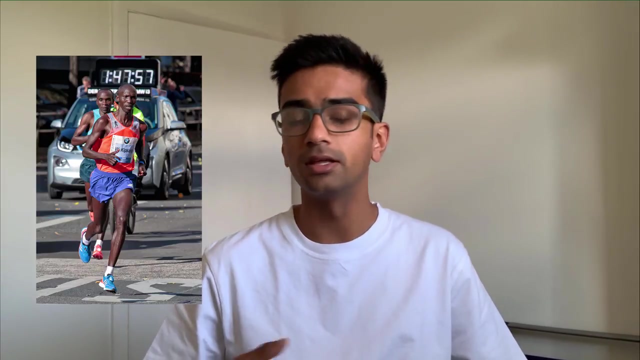 this is already a good indicator that aerospace engineering is the degree for you. If you intend to make your passion and interest into your profession, then you'll need an aerospace engineering degree to work on aircraft and spacecraft. Also, studying at university is more so a marathon than a sprint, and if you have a deep rooted connection to the topic that you're studying, 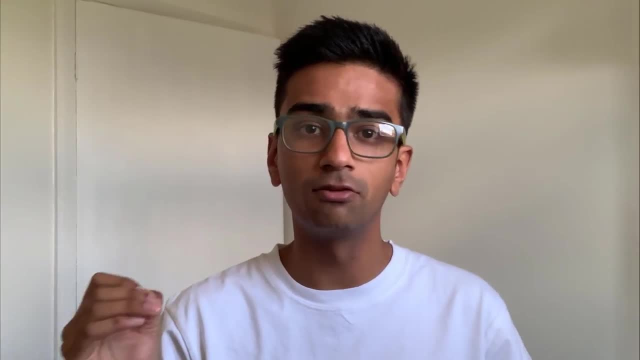 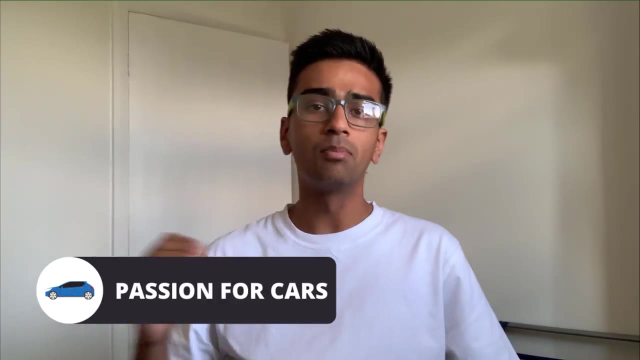 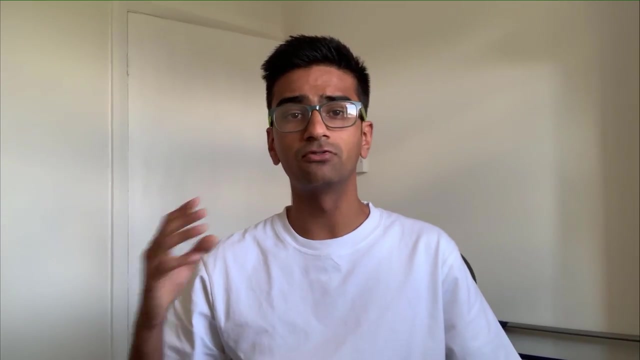 then it makes it so much more easier to power through the tough times during your degree because you have something deeper to connect to and think. you know what I'm going to get this degree. Point two: you have an interest in cars. If aircraft and spacecraft is not your cup of tea, but cars and motorsports are, then aerospace engineering. 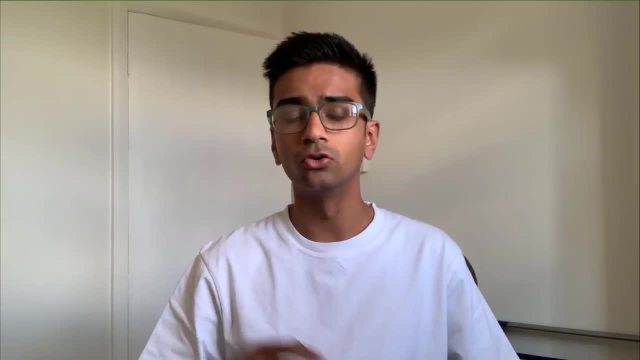 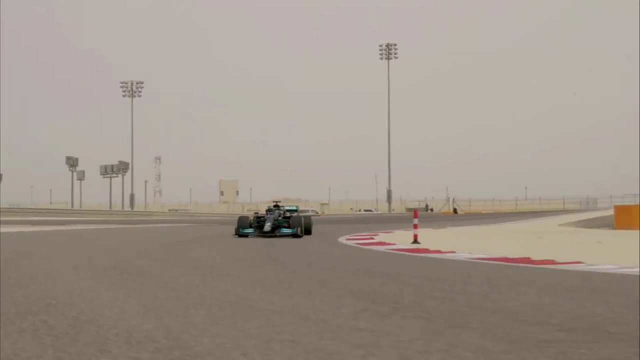 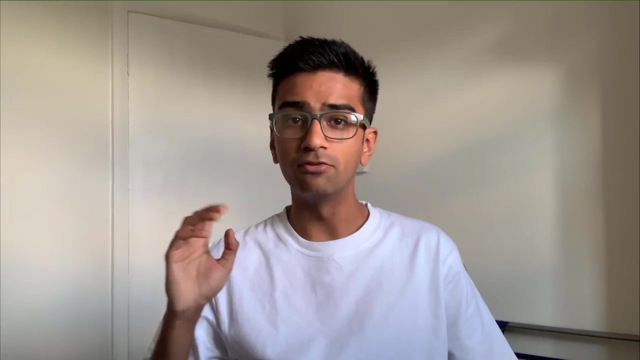 may still be the degree for you. The motorsport and automotive industry hire many aerospace engineers due to their specialized skills in aerodynamics. Formula One is a great example where the work of the aerodynamicists greatly impacts the success of the team. Therefore, if you have an 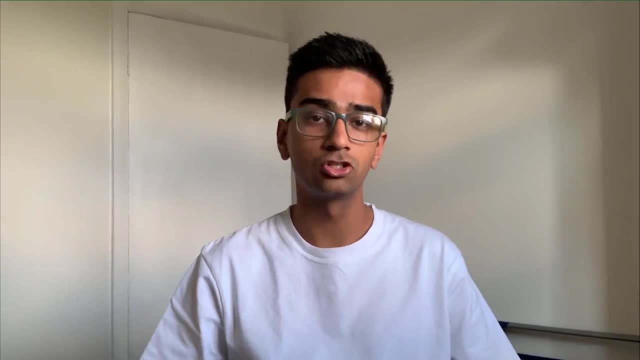 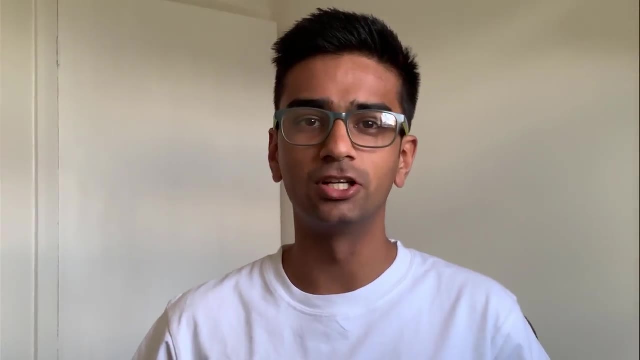 interest in motorsports and automotive and that's the industry you want to go into after university, then aerospace engineering is the degree for you. Point three: you have a passion for aerodynamics. If an aerobatic engineer needs to work in the field of aerobatics, he wants to study. 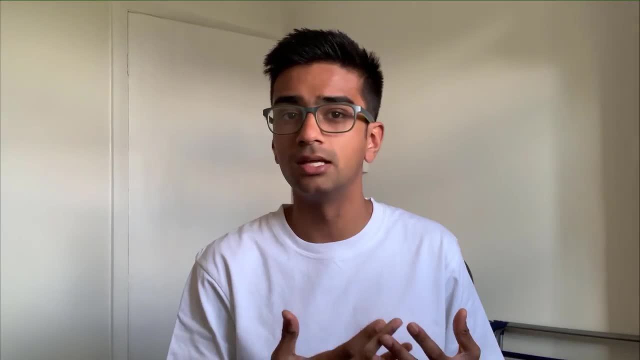 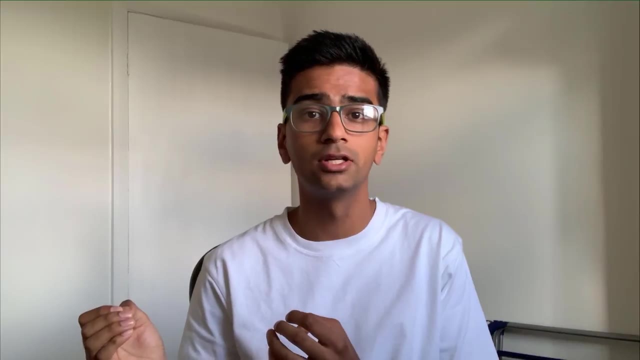 he's going to know a lot about aerobatic engineering, and so he will bring you a specific skill set that will help you to keep your spirit up. If you're more into aerobatic engineering, then aerospace engineering is a great choice for you. So if you study aerospace engineering and then 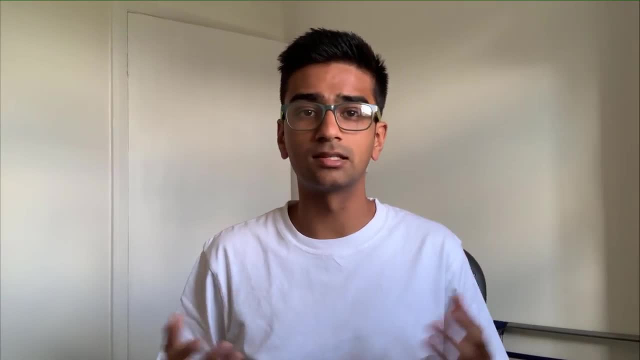 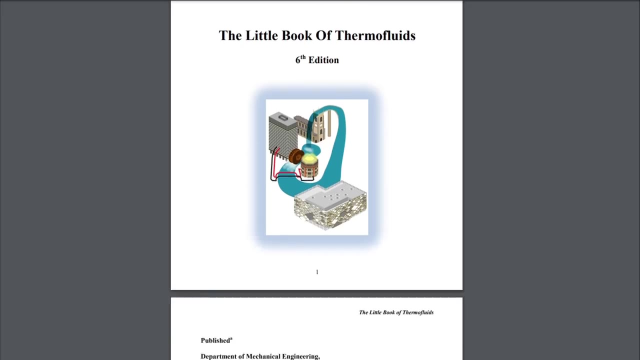 If you've excelled in maths and physics whilst at school, then you have an excellent foundation to do well in your aerospace engineering degree. Aerospace engineering is a very maths heavy subject, and if you are able to understand these complex calculations then you'll have a good 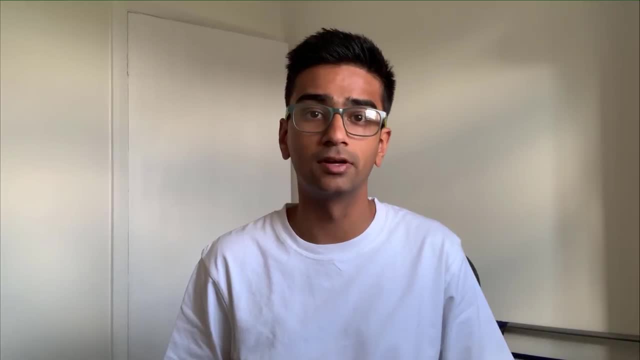 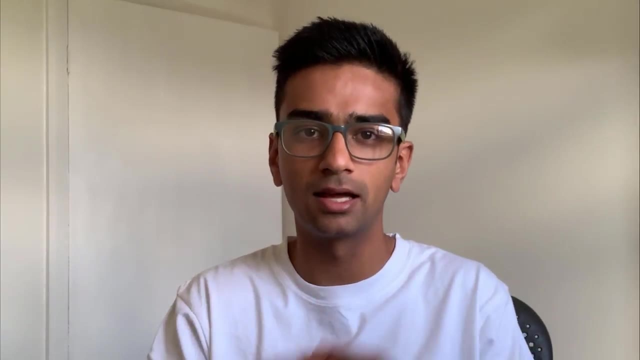 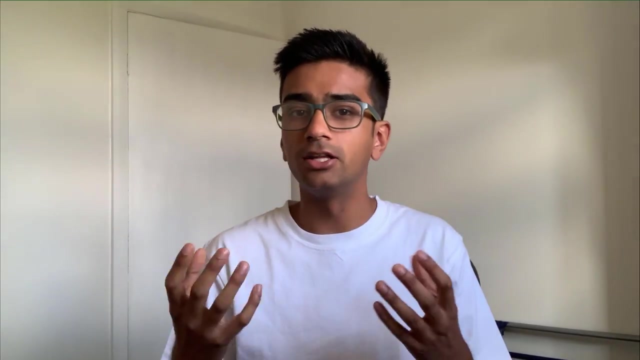 chance of getting a good grade in your engineering degree. Food mechanics and thermodynamics are two of the juggernauts when it comes to maths content in the aerospace engineering discipline. These two are pretty much core subjects in the aerospace engineering degree and you will experience them. 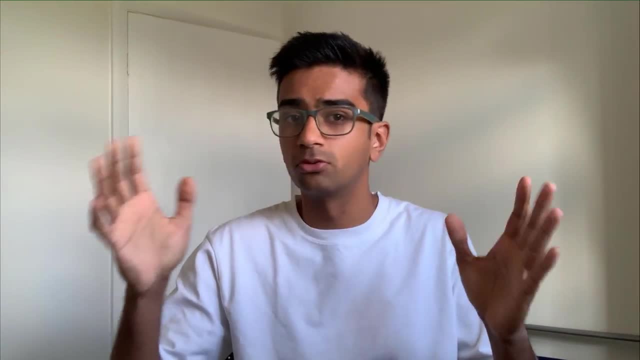 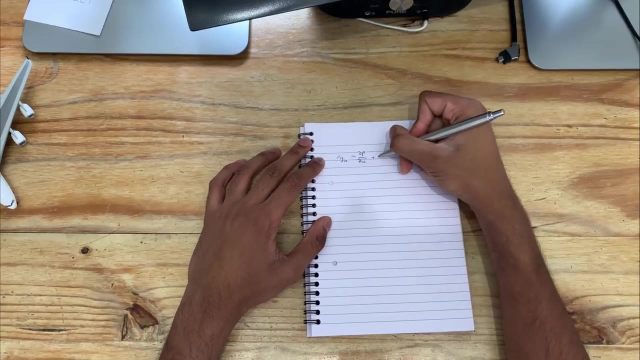 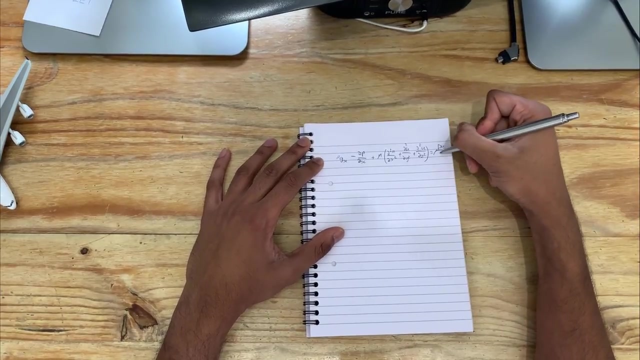 throughout your years, right from first year to your fourth or third year, depending on how long your course is, Since these two major subjects are unavoidable throughout your aerospace degree and they are quite maths intensive. that's why I think, if you're good and have excelled at maths, 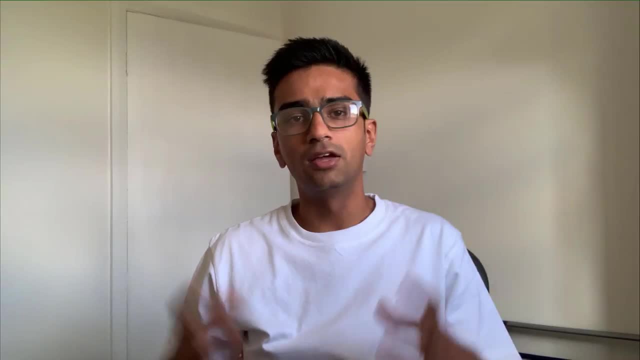 in school, you should choose to study aerospace engineering. If you want to know what sort of grades you should be getting in school, then you should go to the aerospace engineering course. If you want to know what sort of grades you should be getting in school for your maths and physics. 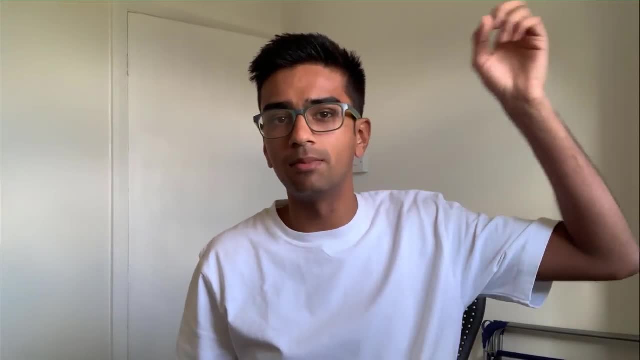 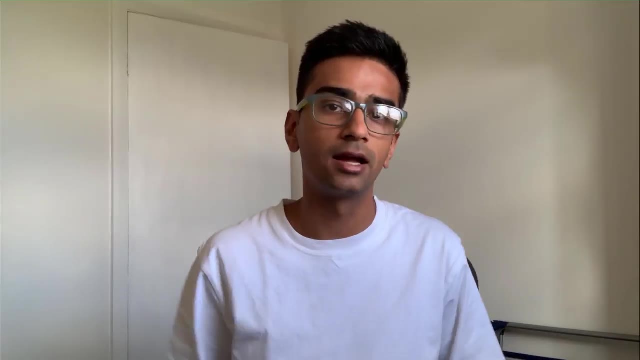 sort of subjects, then click the link above. There's a video I made. I don't know which side it'll appear, but it's talking about what I studied in school and what sort of grades you should be expecting to get to do well in university. Point number four: You enjoy making physical things. If you 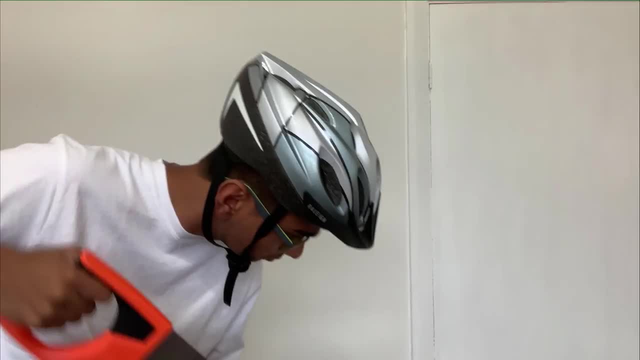 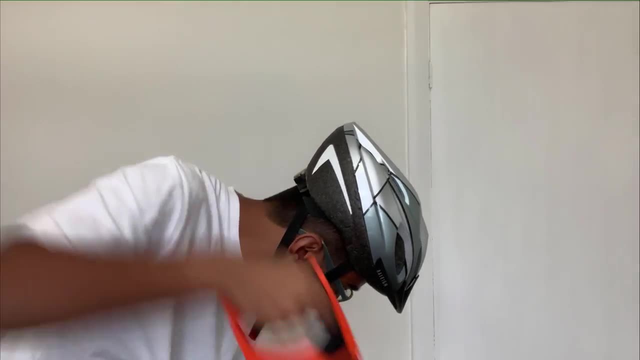 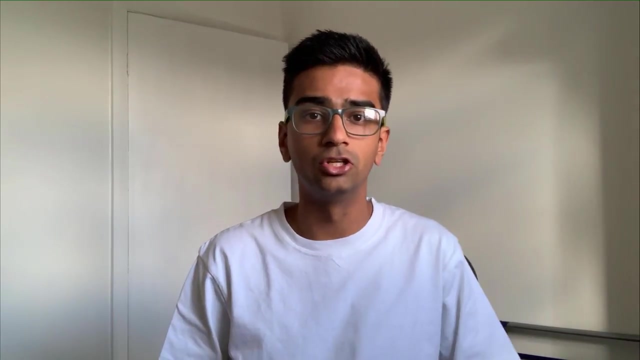 enjoy building physical things- for example, I don't know random DIY in your house to building bikes- then aerospace engineering may be the degree for you. Aerospace engineering is all about building physical things like planes, rockets, cars and even other things like renewable energy, wind turbines. 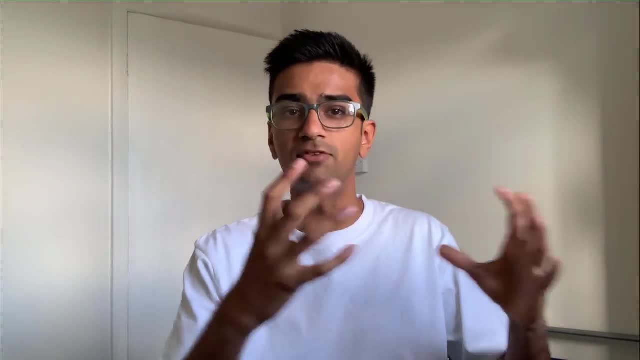 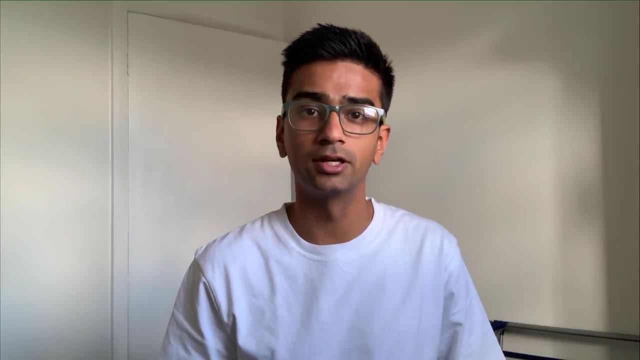 So if you're someone that enjoys the feeling of making a physical thing and then seeing it in the real world and touching it, then aerospace engineering could be what you're looking for. Okay, in reality, as an engineer, you're not going to be building physical things with your hands. 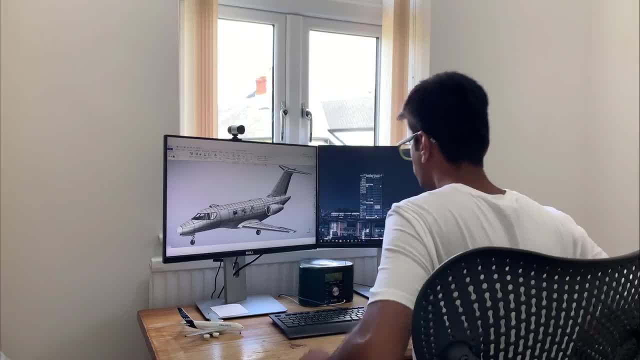 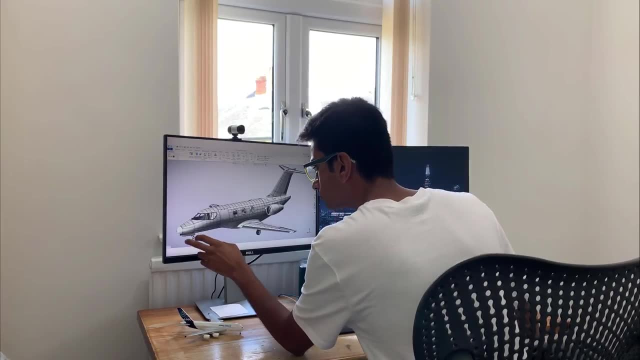 like every day, The reality of being an engineer is that you'd be working with tools on a computer, whether it be computer-aided design or computational fluid dynamics- but the fundamental thing is you're working towards building something that is physical. and even though you are working, 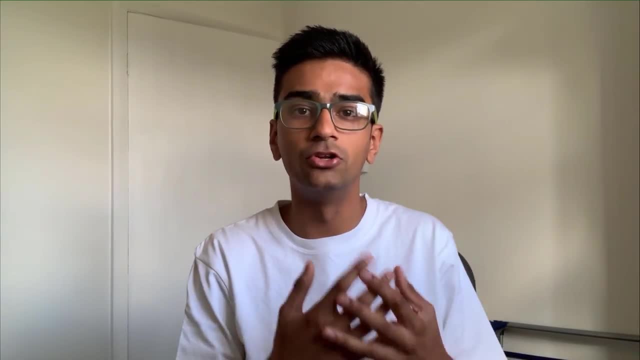 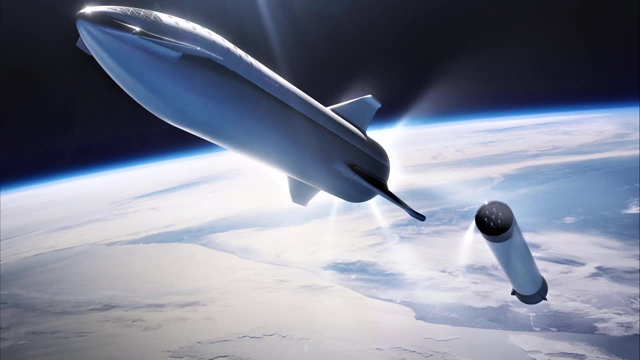 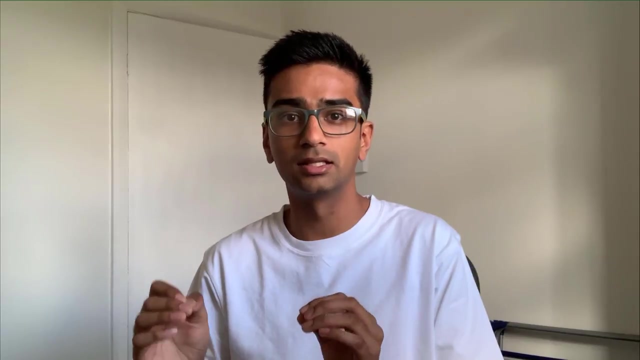 behind a computer screen, I still think there's that excitement of knowing that you're working on building the next generation fighter jet rocket or the latest and most quickest Formula One car. So, ultimately, even though you are at desk, you still know that you're building something that.